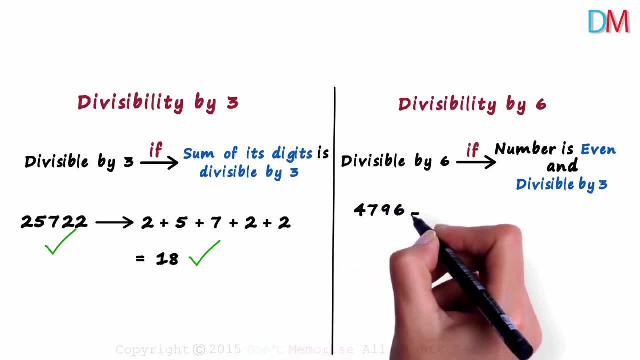 The first one is 479,623.. Is this number even? Since the last digit is not divisible by 2, this number is not divisible by 2.. Hence, this number is not even, So we don't need to check for the other condition here. 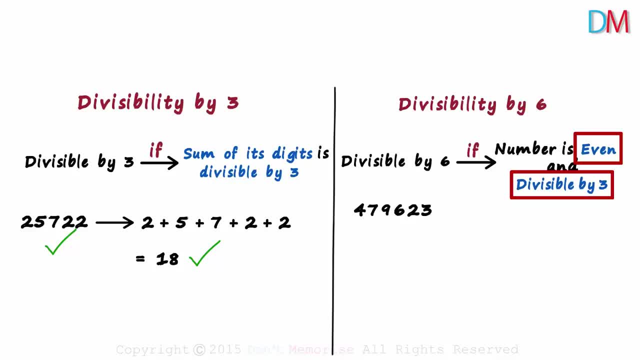 Even if one of them is not satisfied, the number will not be divisible by 6.. Here it's not even and hence will not be divisible by 6.. Consider 190,116.. This number is divisible by 2, as the last digit is divisible by 2.. 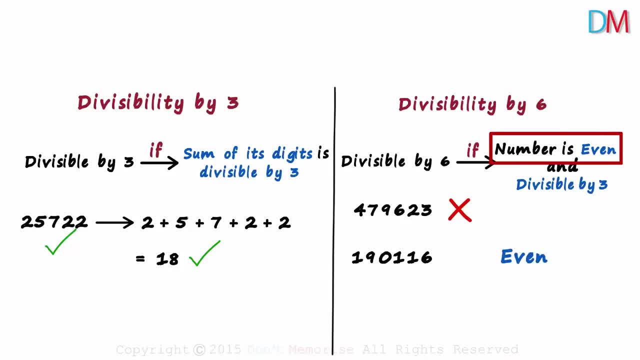 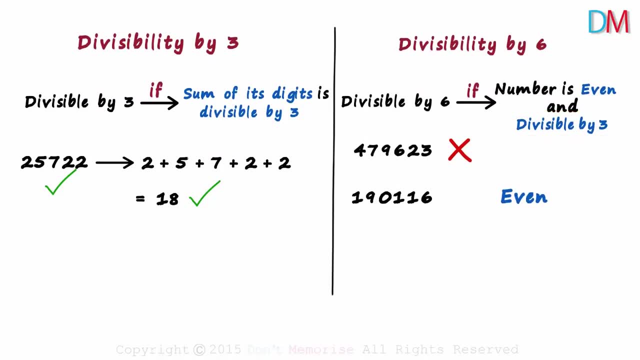 Hence it's even The first condition is satisfied. Now we check for the second condition. We check if it is divisible by 3.. A number is divisible by 3, if the sum of its digits is divisible by 3.. So we find out the sum of the digits. 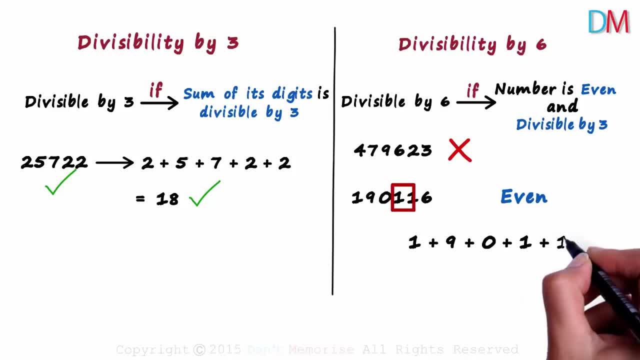 1 plus 9 plus 0 plus 1 plus 1 plus 6.. 1 plus 9 is 10 plus 2 is 12 plus 6 gives us 18. The sum equals 18.. So it is also divisible by 3.. 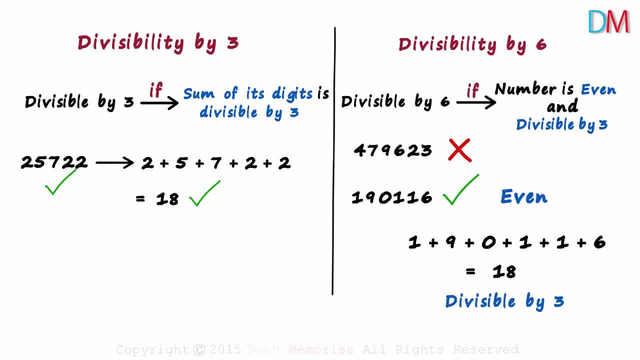 Hence, this number is divisible by 6.. Now we come to the final divisibility test of this video. The test for divisibility by 9, is similar to that of the test for divisibility by 3.. A number is divisible by 9,. 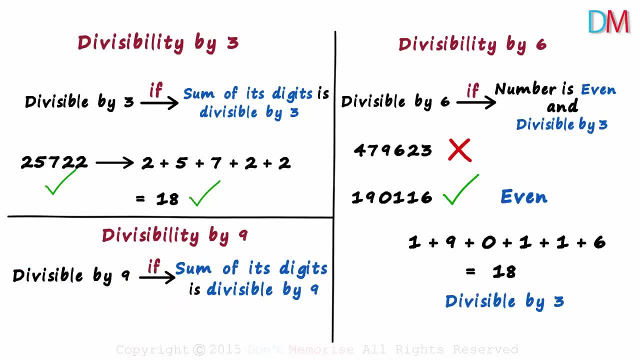 if the sum of its digits is divisible by 9.. Is 2,479,401 divisible by 9?? The sum of the digits equals 27.. Since 27 is divisible by 9, this number will also be divisible by 9..